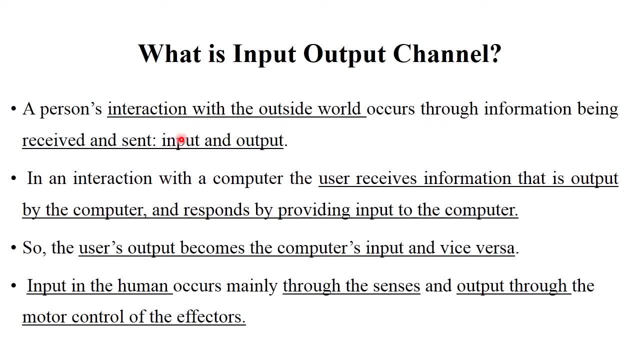 Some speech out loud with the outside the world occur through information being received and sent. This is called as Input and Output, Clear. If you're interaction with the Computer, user receives information that is output by the computer and responds by providing the input to the computer. 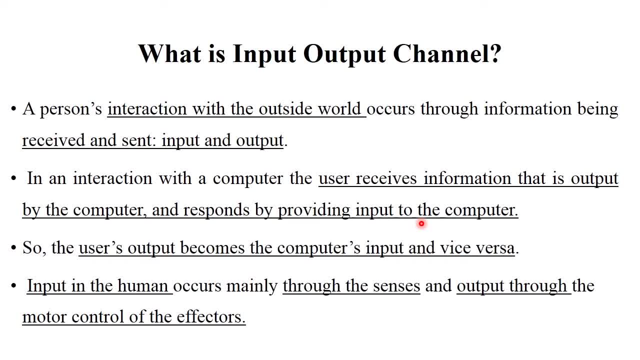 We provide different types of Input to the computer: in the form by using the keyboard Right, And computer gives the proper output through the information or through the screen. Okay, Computer's output becomes computer's input and vice versa. Input in the human occurs mainly through the sense and output through the motor control. 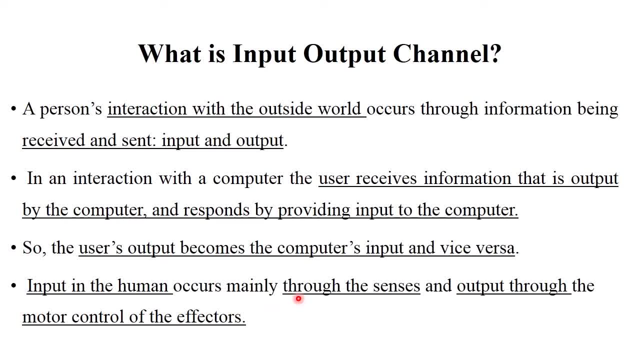 of the effectors: Right When you provide a particular input to the computer by using keyboard. Right. So keyboard is a part of the computer, But what is? which type of sense is used? You used your finger for typing purpose, Okay, 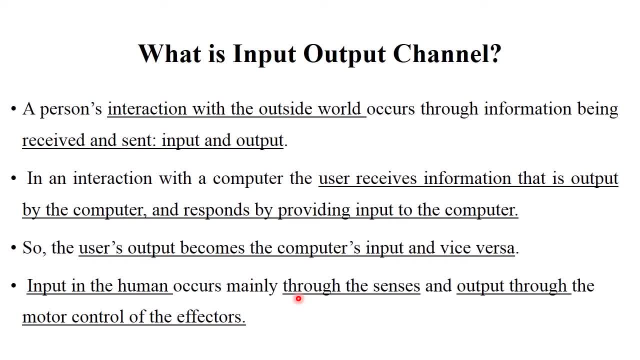 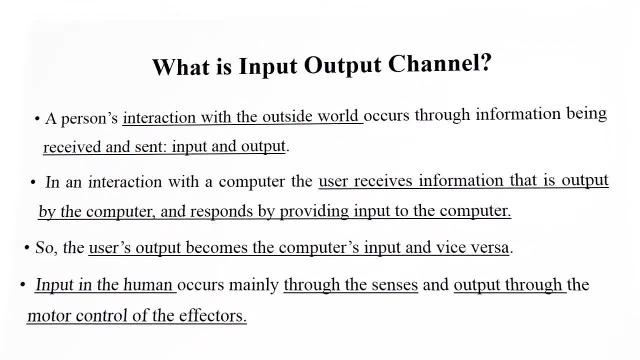 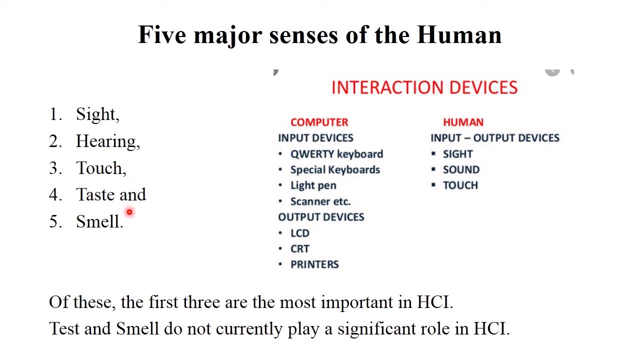 So you provide the input by using your input channel. that is sense, or that is fingers Clear. So this is the concept of input output channel. Okay, Next, Five major senses of human, that is, sight, hearing, touch, taste and smell. 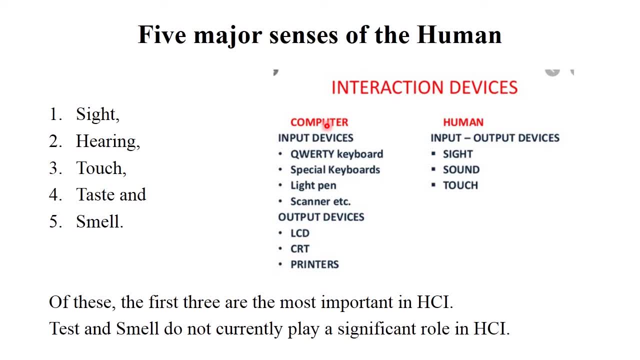 Okay, There are interaction devices. So computer's input device is keyboard, special keyboards, light pin scanner, etc. And output device of computers are LCD, CRT printers, etc. But what is the input, Input? output devices of human are sight, sound and touch. 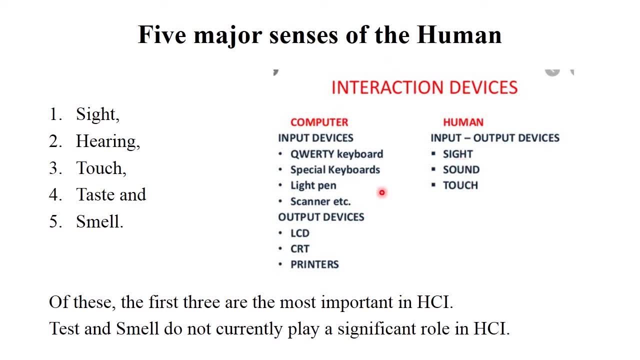 Okay, So this is called as human computer interaction by using interactive devices, Using input and output devices. Clear, Okay. So of these first three are the most important in human computer interaction, That is, sight, hearing and touch. But taste and smell do not currently play a significant role in human computer interactions. 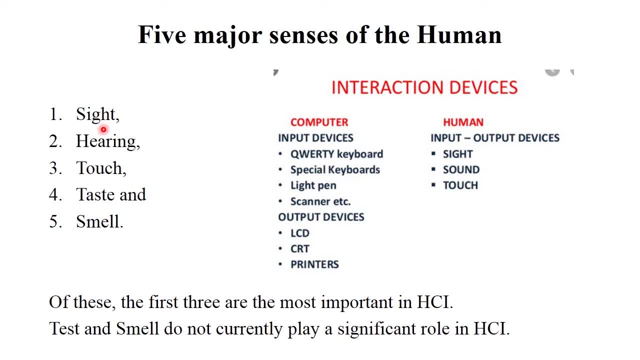 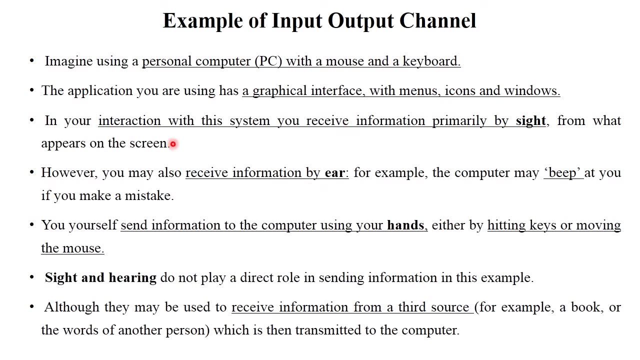 Clear. So let's see one by one, That is how sight, hearing and touch, these kind of human senses, are work in human computer interaction. Okay, Next Let's see first the examples of input output channel. Okay, Just imagine that using your personal computer with mouse and keyboard. 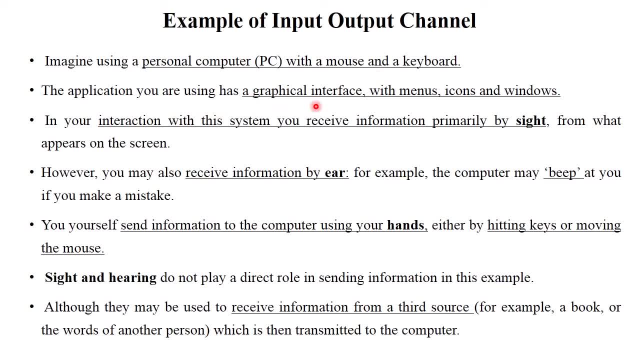 Okay, The applications you are using has a graphical interface with menus, icons and windows, etc. If you interaction with this system, you receive information primarily by sight. Sight means eye region. Okay, From what you appears on the screen: Okay, You will see each and every information on the screen by using your eyes or using your 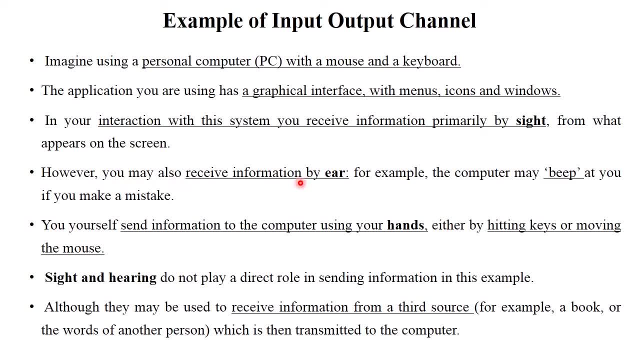 sights- Okay. However, you may also receive information by the ear, For example. computers may beep at you if you make mistakes, Right? You yourself send information to the computer- Okay. You send information to the computers using your hands, Either by hitting the keys or moving the mouse, etc. 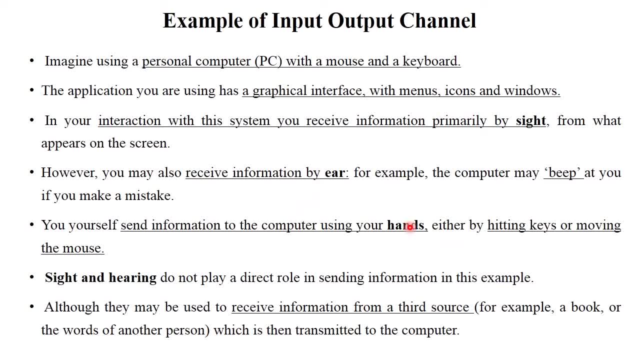 So in this way, the sight, ear and hands, these kinds of input output channel you used with computers, Sight and hearing- do not play a direct role in sending information in this example, Okay, Although they may be used to receive information from the third source. 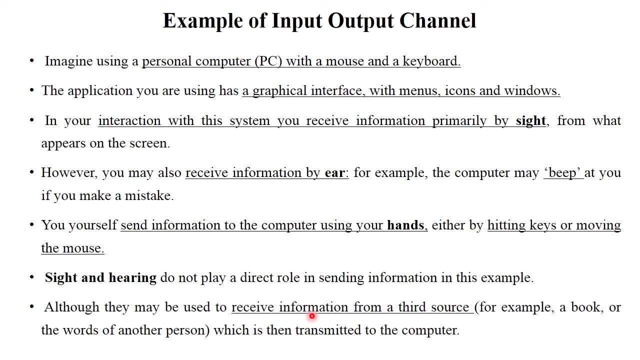 For example, book the word or another person Clear. So in this way, sight, ear and hands: Sights for visionary purpose, ear for receive the information and hands for sending the information to the computer. Okay, So this is the example of input output channel, how human use their senses for handling the 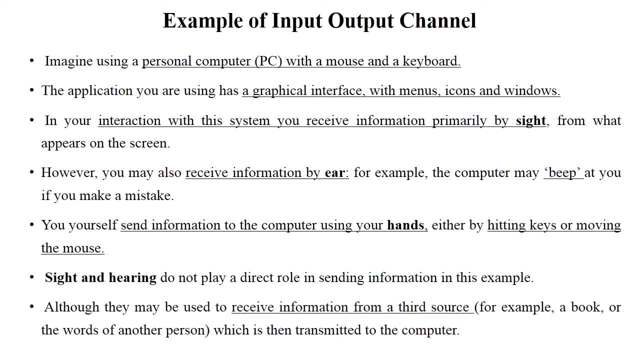 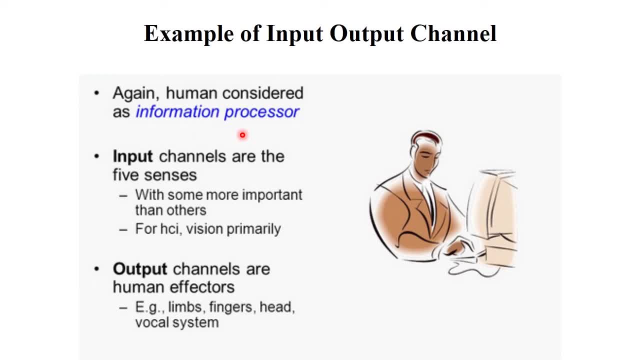 computers Clear. Okay. Next, This is another example of input output channel, Again human considered as information processor. Input channels are the five senses, with some more important than others. Okay, For SCI, vision is preliminary purpose. Vision is one of the most important part in human computer interaction. 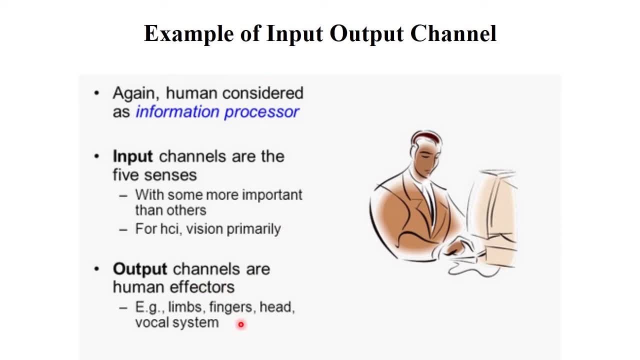 Okay, Then output channels are human effectors like fingers, head, vocal system lines, etc. Okay, By using your vision, you can catch the information and store this, all the information, in your brain. Okay, This is one of the most important part, that is, input- output channel. 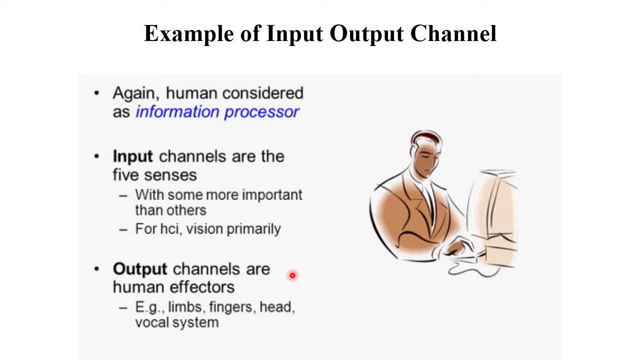 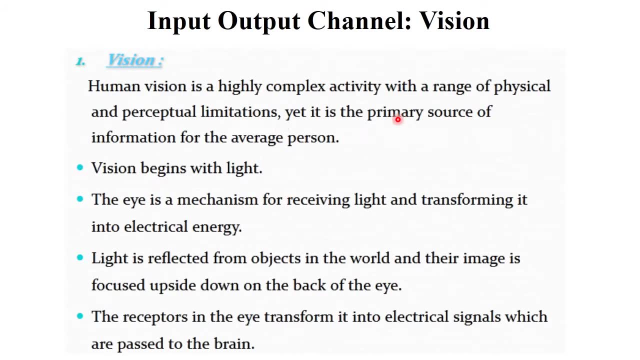 This all the input outputs we use in our daily life. Okay, Next Input output channel, or first input output channel, is vision. So what is mean by vision? Human vision is highly complex activity with a range of physical and perceptual limitations. 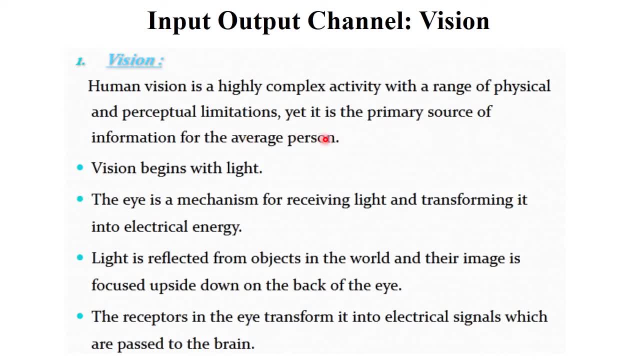 Yet it is the primary source of information for the average person. Okay, Vision begins with the light. The eye is the mechanism for receiving light and transforming it into electrical energy. Light is reflected from the objects in the world and their image is focused upside down. 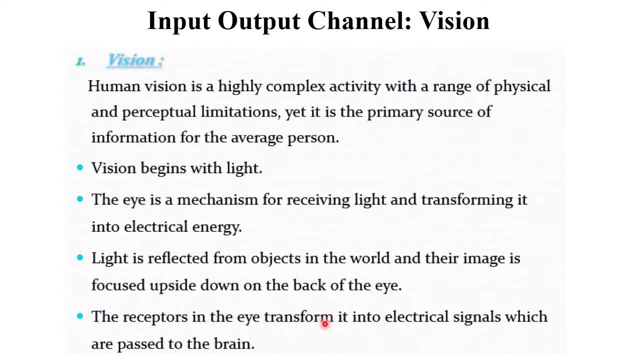 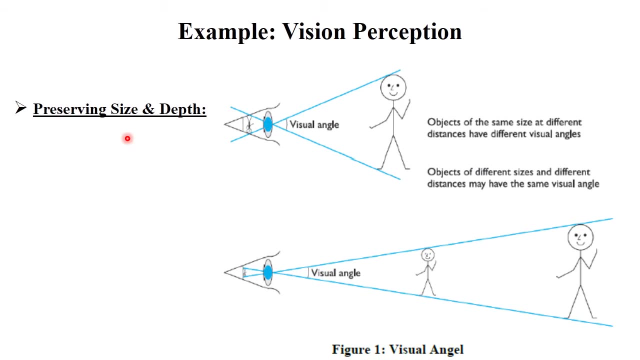 on the back of the eye. The respectors in the eye transform it into electrical signals which are passed to the brain. In this way, visions are work, Okay. Next, This is the example of vision perception: Okay. This example shows preserving size and depth. 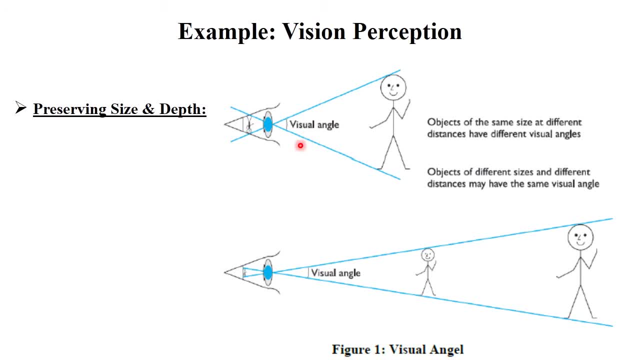 See here: Objects of the same size at different distance have different visual angles. And objects of different size and different distance may have same visual angles. Okay, Suppose this is your visual angle and this person is placed here. The distance is very less. 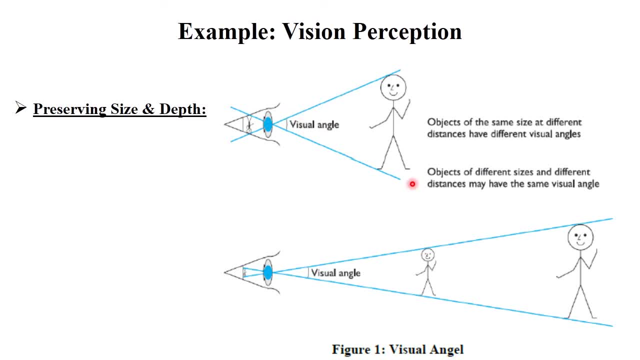 Okay, So your visual angle works in this way. Okay, But same This object going to far away from your visual angle. Okay, The distance is more as compared to this distance, So your visual angle see this object in this way. 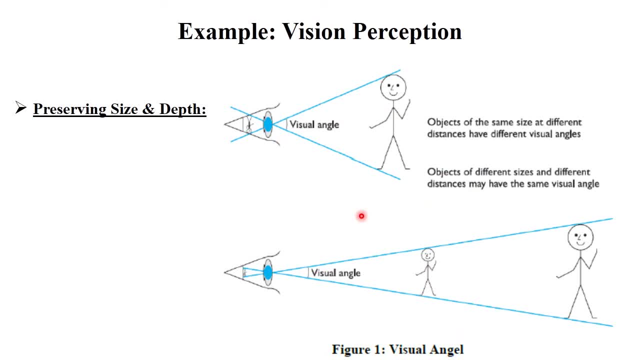 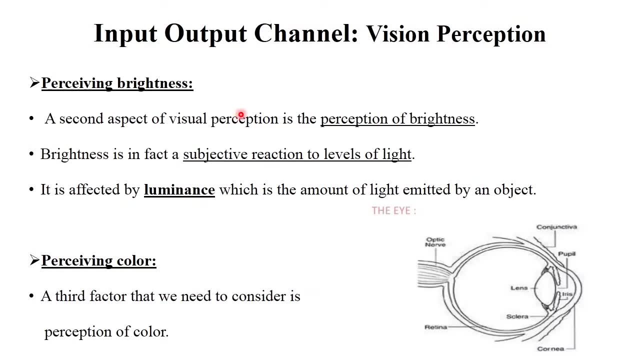 Clear. So this is called as visual perceptions, which is mostly used in human computer interactions. Okay, Next, Next. So vision perception is preserving brightness. You can control your mobile brightness or computer's brightness by using some keys. The second aspect of visual perception is perceptions of brightness. 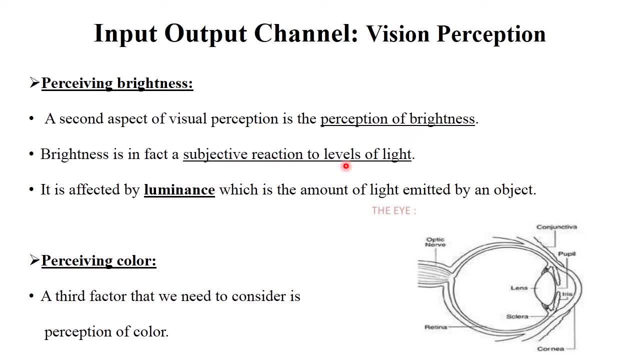 Brightness is in a fact of subjective reaction to levels of light. Okay, It is affected by the luminance, which is the amount of light emitted by an object. Okay, So brightness is different for each and every visual perceptions of persons. Each and every persons require different brightness of computers or the mobiles. 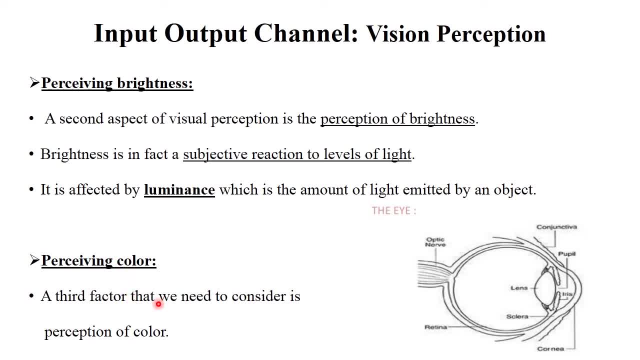 Right. And the last one is preserving color, A third factor that we need to consider: perceptions of color. By using your vision, You can identify the colors of each and every word, each and every object or the systems Right. So this is called as vision perceptions. 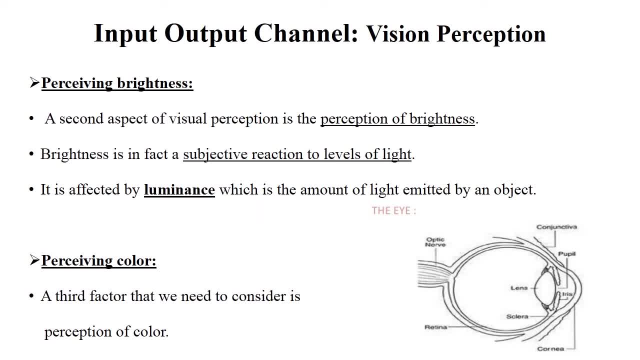 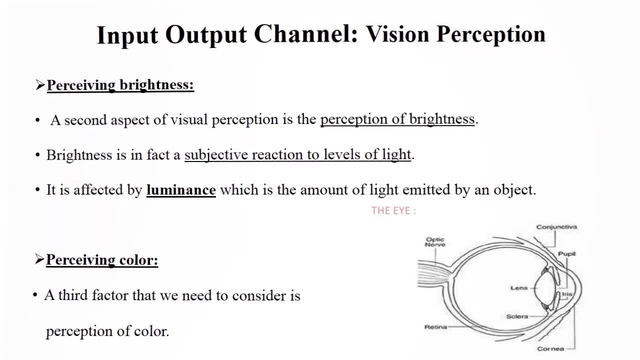 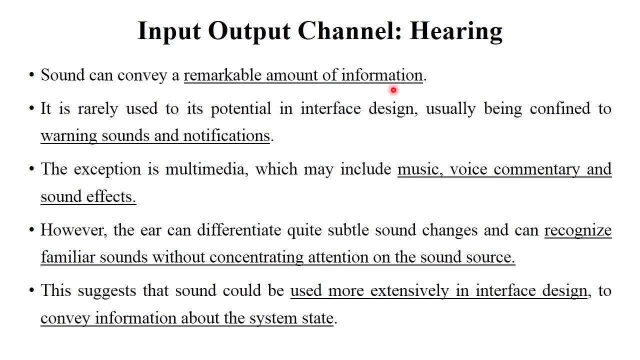 That is, preserving size, preserving depth, preserving brightness and preserving color. This is called as vision perceptions Clear. Okay. Next Input output channel is hearing. Sound can convey a remarkable amount of information. It is really used to potential in interface design. 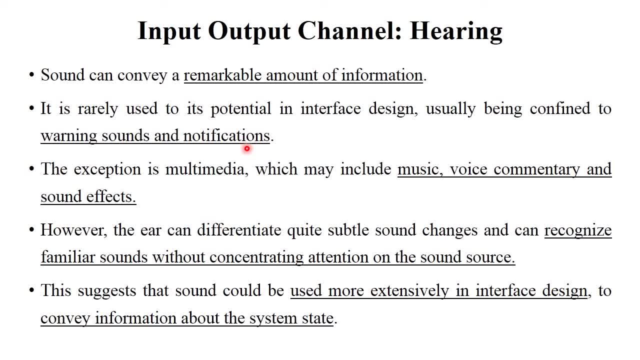 Usually being conformed to warning sounds and notification. Okay, When systems can provide a particular notification beep or sound, you can hear this sound by using your ears Right. So the exception is multimedia, which may includes music, voice commentary and sound. 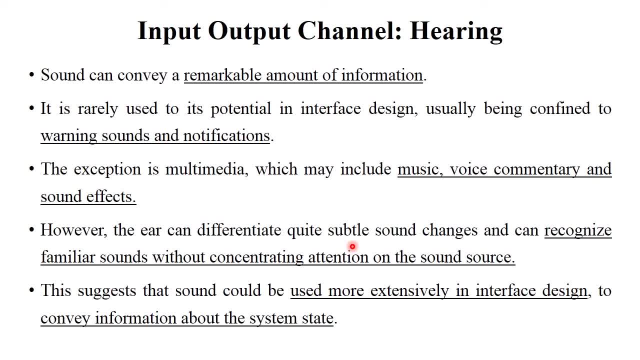 effects. However, the ear can differentiate quite suitable sound changes and also recognize familiar sounds without concentrating attention on the sound source. Okay, There are some sounds you are familiar of this. Okay, When you don't see that particular object, but you identify the sounds. 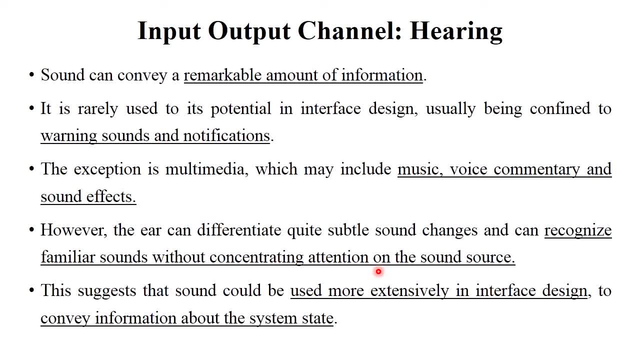 Okay, Because you are familiar with that sound. This is the input output channel hearing. This suggests that sound could be used more extensively in interface design to convey information about the system state Okay, If system shows the warning, you identify that particular sound. 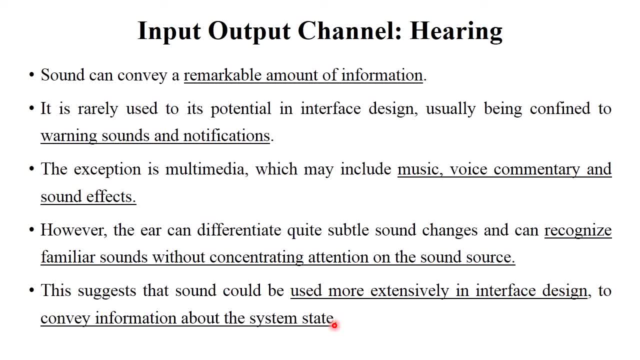 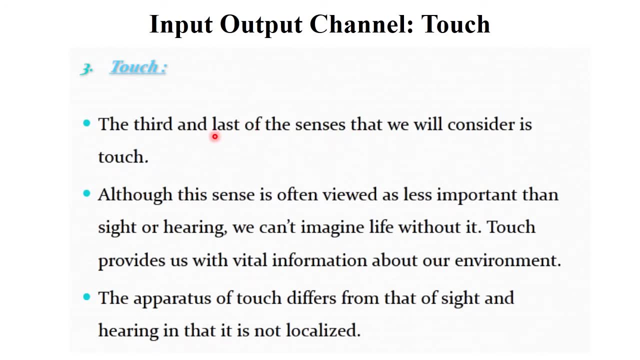 If system shows the beep Or generate a beep, Then you can identify the system state Right. So this is the work of hearing. input output channel Clear. Okay, Next. Next output channel is touch. This is the third and last of the sense that will be considered is touch. 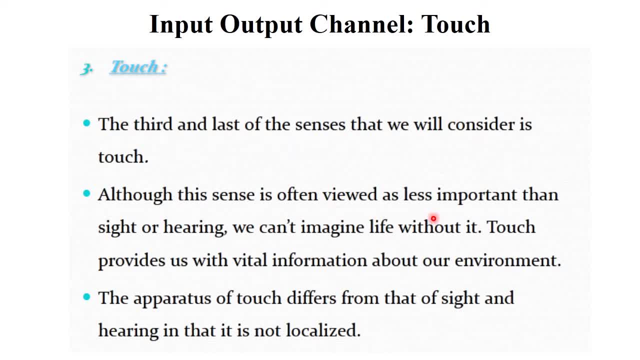 Although this sense is often viewed as less important than sight. of hearing, Okay. We can't imagine life without it. Touch provides us vital information about our environment. The apparatus of touch differ from that of sight and hearing. is that not localized? Okay. 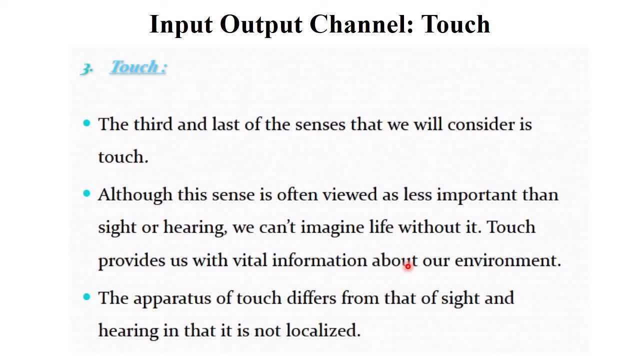 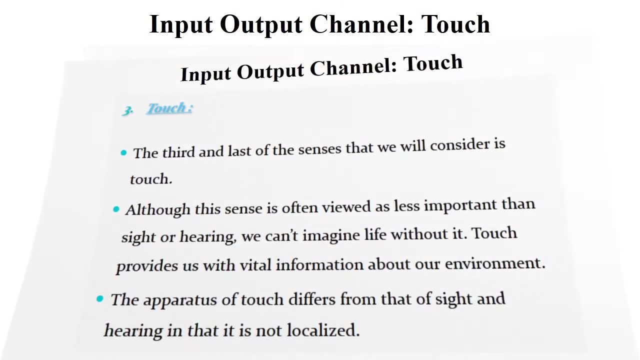 By using touch you can identify the keyboard, mouse, different types of keys, etc. Okay, So touch is also one of the important part, But the more important is sight and hearing. Okay, Next, In input output channel, touch.